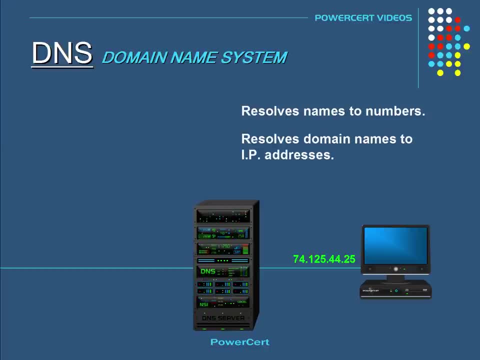 You can just type in the IP address instead, if you already knew what the IP address was. But since we are not accustomed to memorizing and dealing with numbers, especially when there are millions of websites on the internet, we can just type in the domain name instead and let DNS convert it to an IP address for us. 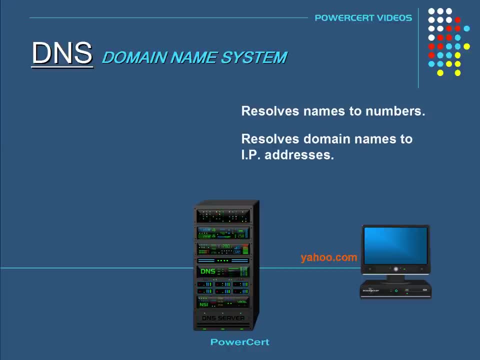 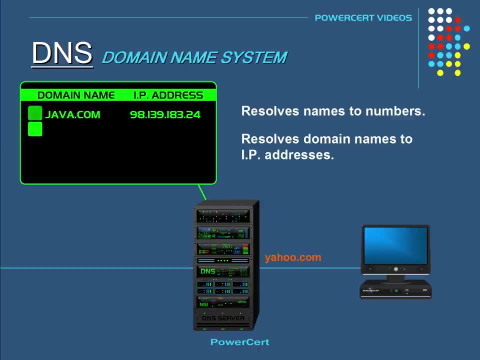 So back to our example. when you type in yahoocom in your web browser, the DNS server will search through its database to find a matching IP address for that domain name And when it finds it, it will resolve that domain name to the IP address of the Yahoo website. 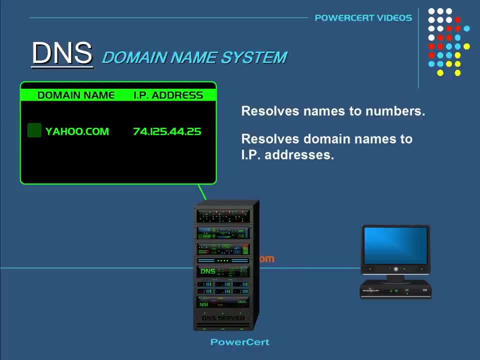 And once that is done then your computer is able to communicate with the Yahoo web server and retrieve the web page. So DNS basically works like a phone book. When you want to find a number, you don't look up the number first, You look up the name first. 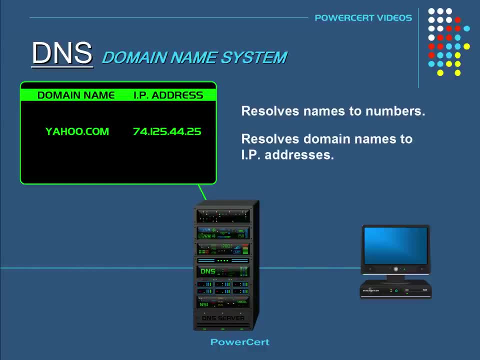 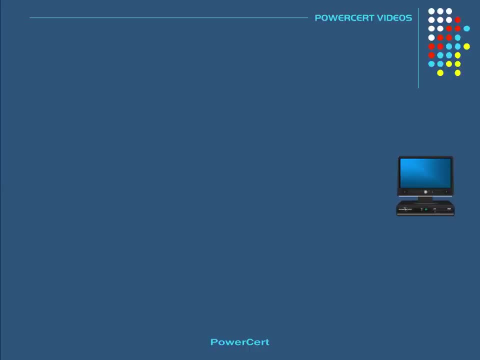 Then it will give you the number. So to break this down into further detail, let's examine the steps that DNS takes. So when you type in yahoocom in your web browser and if your web browser or operating system can't find the IP address in its own cache memory, 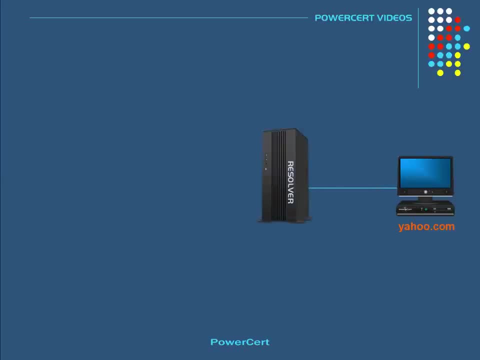 it will send the query to the next level, to what is called the resolver server. The resolver server is basically your ISP or internet service provider, So when the resolver receives the query, it will check its own cache memory to find an IP address for yahoocom and. 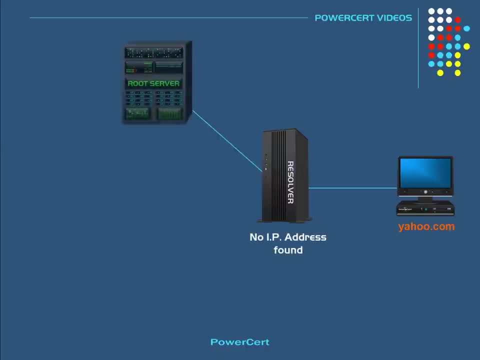 if it can't find it, it will send the query to the next level, which is the root server. The root servers are the top or the root of a DNS hierarchy. There are 13 sets of these root servers and they are strategically placed around the world and they are operated by 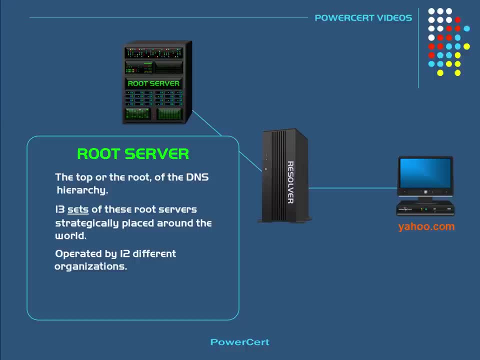 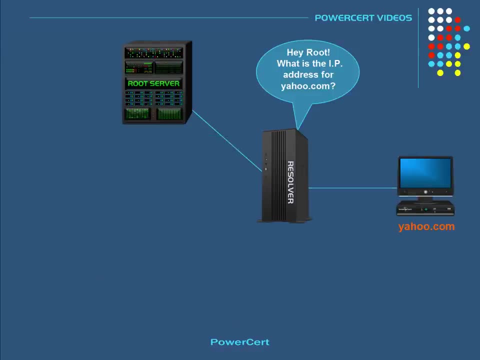 12 different organizations and each set of these root servers has their own unique IP address. So when a root server receives the query for the IP address for yahoocom, The root server is not going to know what the IP address is, But the root server does know where to send the resolver to help it find the IP address.